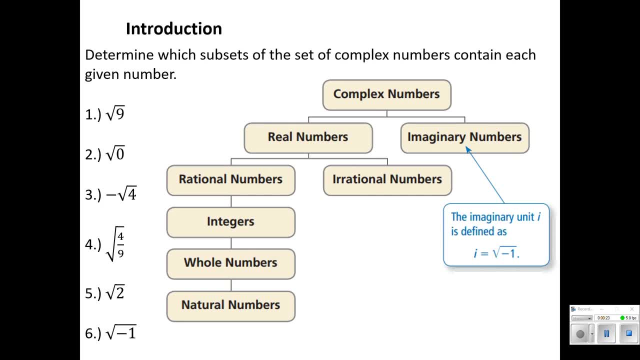 set of complex numbers contain each given number. So I'd like you to pause the video and see if you can't make some predictions on which of those six numbers given at the left belong to which subsets of this set of complex numbers. So pause the video and I'll check back in a few seconds. 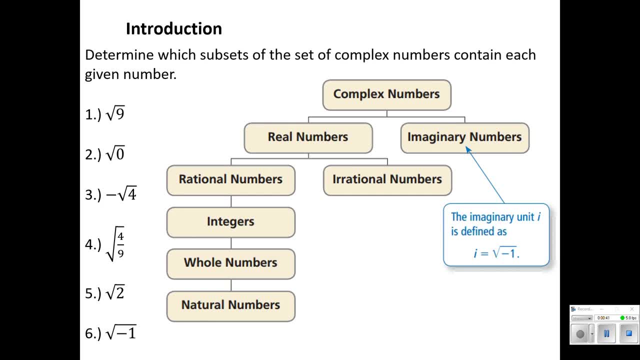 to go through this. Okay, well, let's have a look. Problem number one or number number one: we've got the square root of nine, which is equal to three or negative three. We've got integers here, and really integers. the positive three would fall. 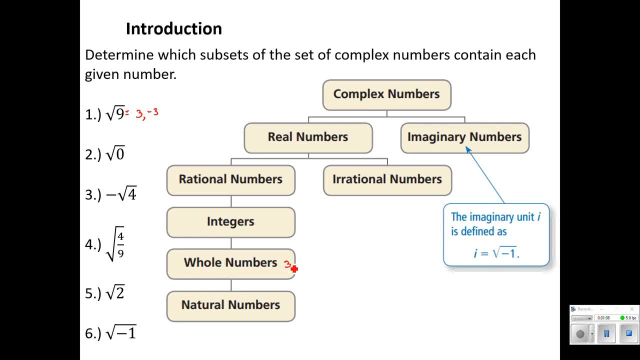 in the whole numbers category and the negative three would fall in the integer category, Remember, natural numbers. that's where, actually, this is a very neat talk to have and I won't take much of your time to do this, but this is kind of the progression of how we developed our numbers. 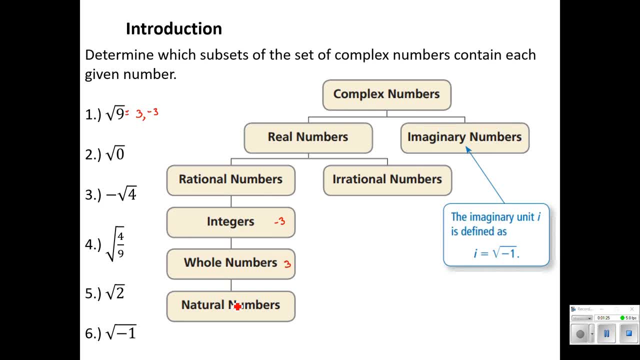 to explain the world around us. So, cavemen counting rocks. they started off by the natural numbers, what we use to count numbers like one, two, three. I have five rocks. Then whole numbers were introduced to include zero. We needed something to represent no rocks. So if I have, 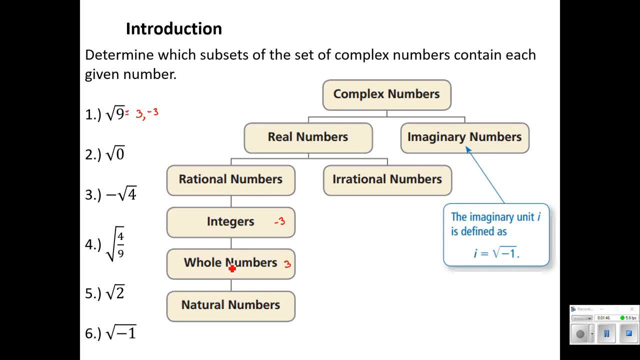 three rocks and you take away those three rocks, then I have zero rocks. Next, as our number system progressed, we developed integers, and this includes negative numbers. So now tax collectors would come around and say: oh, you owe me three gold pieces, three doubloons or something, and you'd say: 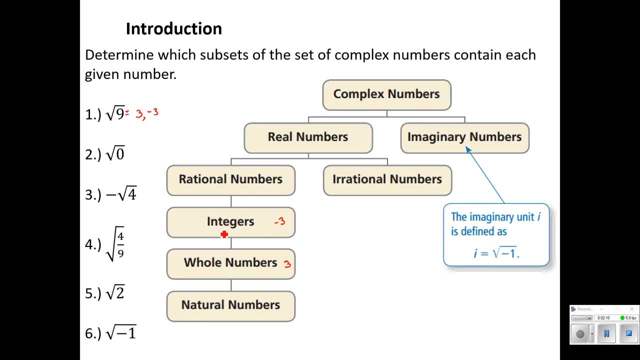 I don't have that. And then if you have two doubloons, then you know that that tax collector is still expecting one. so you technically have negative one doubloons or whatever. After that rational numbers were established. These are your fractions and we use these to describe, obviously, parts of a whole piece. So 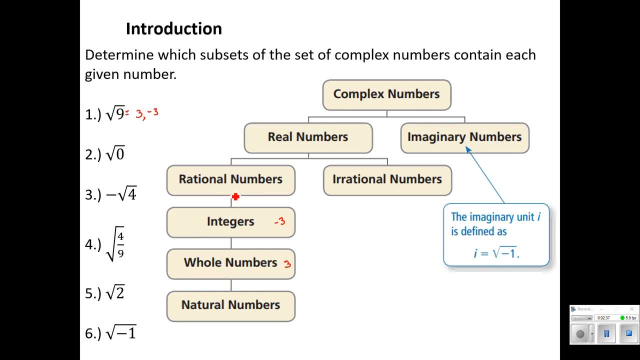 you know I have half a rock, or you know my land is one half of your land, something like that. Rational numbers include those fractions. to break apart numbers using division, divide them up. Okay, All of this got grouped under the. 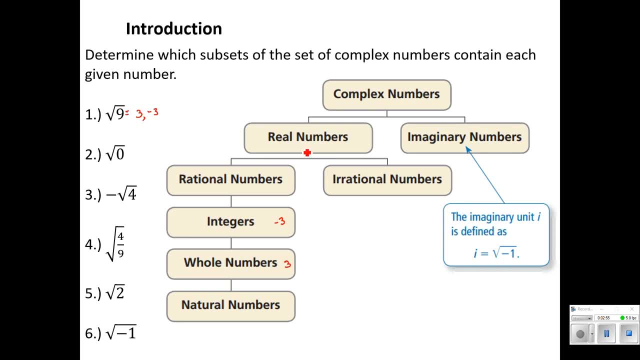 under the classification of real numbers, numbers that we can work with and see and evaluate. We also include irrational numbers here. These are numbers like e and pi that were used in or like square root of seven. A lot of these emerged from geometric observations in, like ancient Greece. 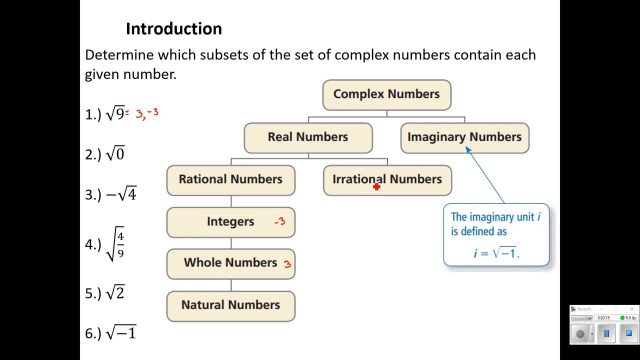 So they're still real numbers, but they are very intricate. They are not decimals, that stop. They can't be expressed as a fraction. Well, what we found? that there were situations where we would need imaginary numbers to kind of fit a need. 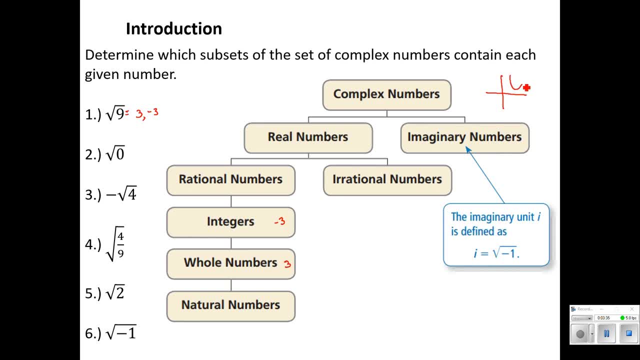 So we saw the situation where we had a parabola that did not intersect the x-axis. That actually has solutions, even though we called solutions x-intercepts- Imaginary numbers kind of fit that need to give every single parabola the two solutions, and that's something we'll explore further in later chapters. 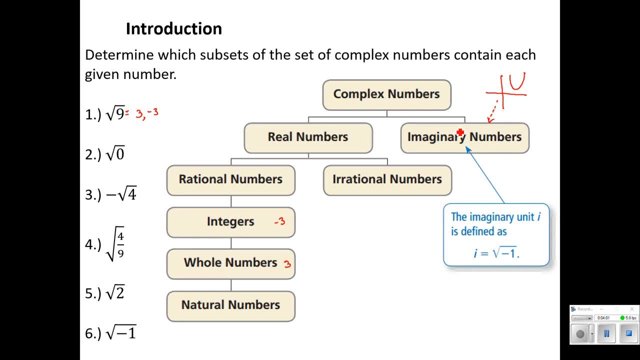 But we needed this set of numbers to kind of establish an ironclad pattern for us. And you can see that imaginary numbers use this variable i to denote a negative underneath the square root. All right, And then all of this falls under the blanket of complex numbers. 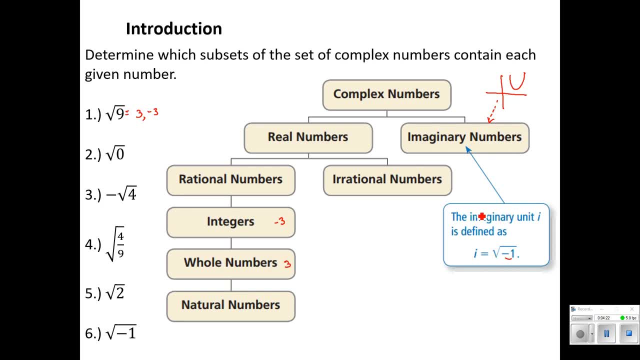 So our entire set of numbers are complex. All right, let's look at number two, the square root of zero. Well, that equals zero And that falls into our whole number category. We have no rocks. Number three: the negative square root of four. 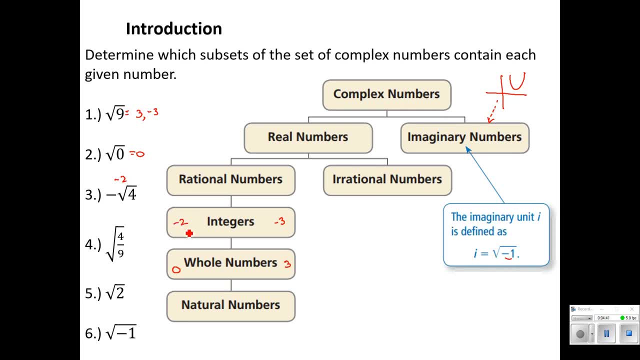 Well, that's negative two And that is an integer Number four, the square root of four ninths. Remember, if we take the square root of a fraction, it's like square rooting the top and square rooting the bottom. So we're going to take the square root of a fraction and square rooting the top and square rooting the bottom. 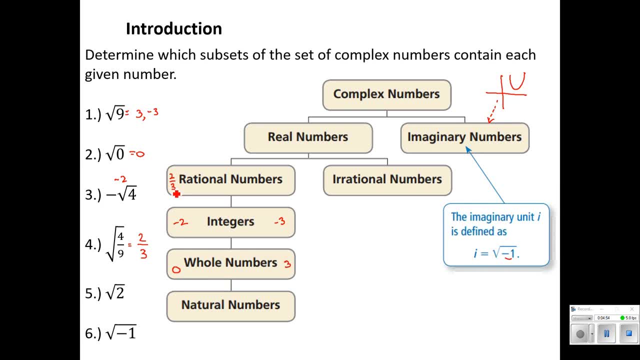 We've got two thirds. That's a fraction that falls in our rational number set, The square root of two. that is a decimal that keeps on going. One point four, one. It does not stop. That is an irrational number. Drove the ancient Greeks mad. 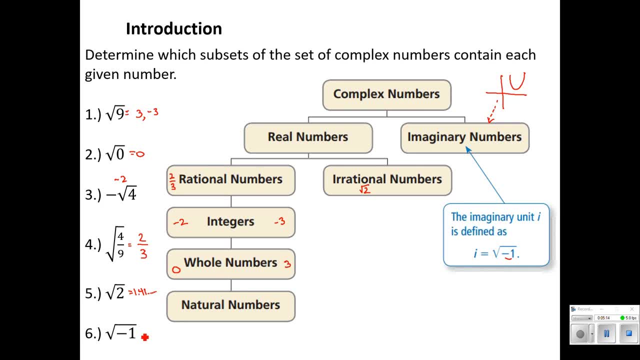 And then, lastly, we have the square root of negative one. Well, that's kind of a dead giveaway. The imaginary unit is defined as the square root of negative one. So that is an imaginary, So that is an imaginary number. This slide, really, this introduction, it was designed primarily just to give us an understanding of vocabulary and classifying all these different types of numbers that exist in our mathematical system. 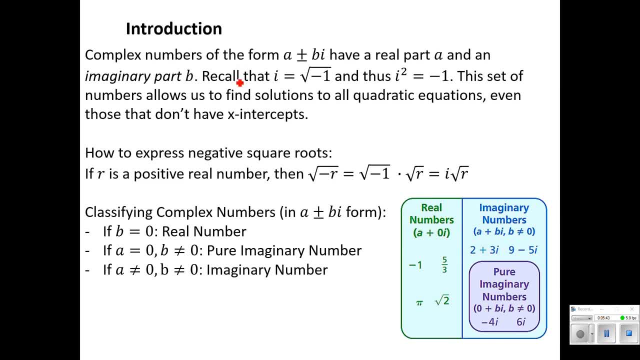 All right. So now that we're talking about complex numbers, how do we classify all these numbers under the same blanket, no matter what subset they fall into? Well, our solutions, and really all of the complex numbers, follow this form: A plus or minus B I. 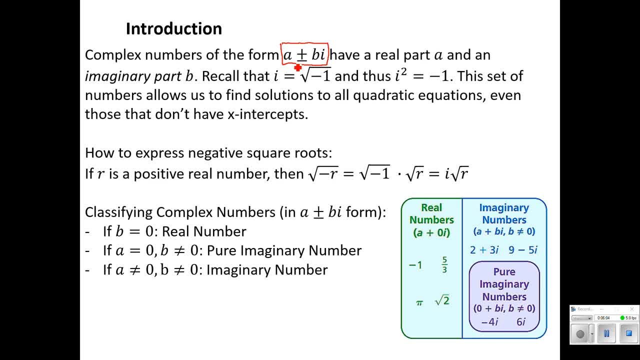 So it looks kind of like an expression instead of an actual number, but it really is a number, And so we want to remember to think of it that way. That is, simply representing a number, even though we see some variables in there. All right, 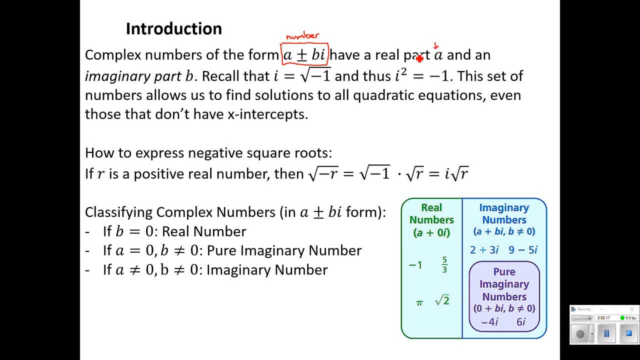 There is a real component to that A and an imaginary part B, So you can see that the real part has No I attached to it, while the imaginary part does have I attached to it. And remember that I is just a placeholder for square rooting a negative. 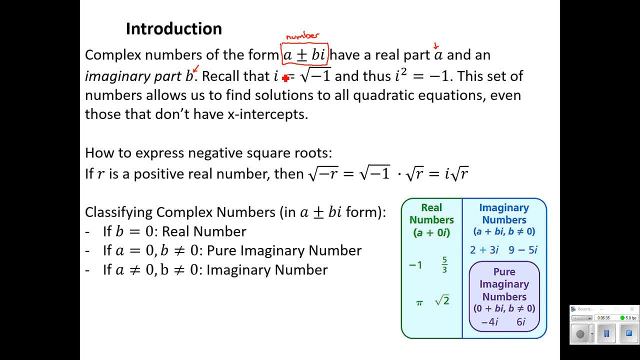 All right. And if we square both sides of that little definition we get: I squared equals negative one, All right. And again, we already talked about having this complete set of numbers allows us to find the solutions to all quadratic equations, even ones that don't have X intercepts. 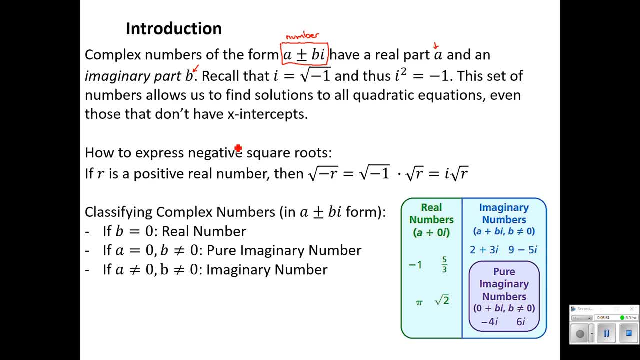 All right, How to simplify negative square roots. if we don't see an I present, but we do have a negative underneath the square root. We know how to handle that now. If R is a positive real number, then the square root of negative R is equal to the square root of negative one times the square root of R. 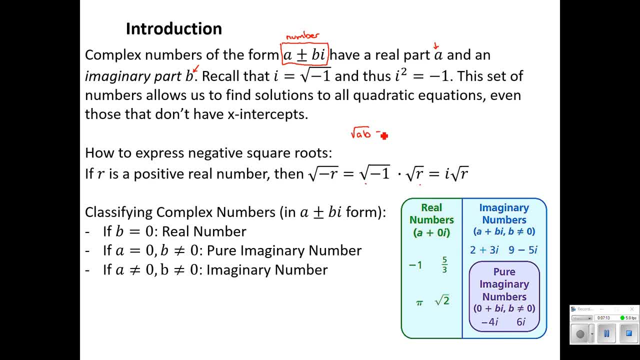 This is called the product property of radicals. If I have two numbers multiplied underneath a square root, then I can separate that and refer to it As the product of two square roots. So that's what we've done here in this first step. 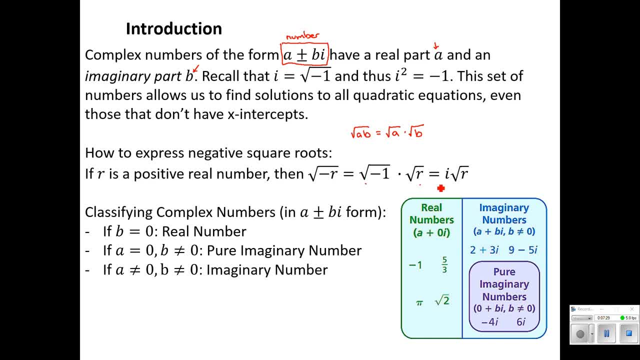 And then, by definition, the square root of negative one is I. So we use that I variable to denote that that's an imaginary part to a number. All right, So the different complex numbers. Well, if we have B equaling zero, that means there is no imaginary part. 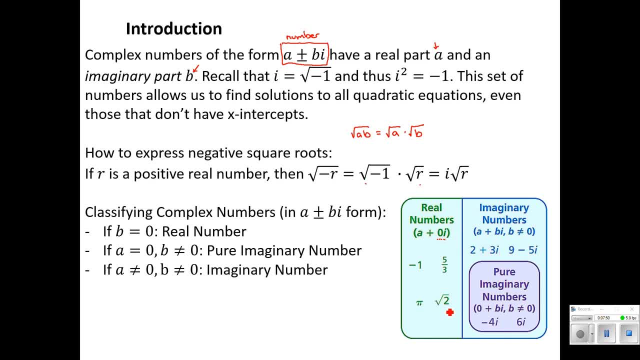 So it's all a real number. And here they've given us some examples of real numbers. If A equals zero and B does not equal zero, we have what are called pure imaginary numbers. Now, there is no real part. Everything is imaginary. 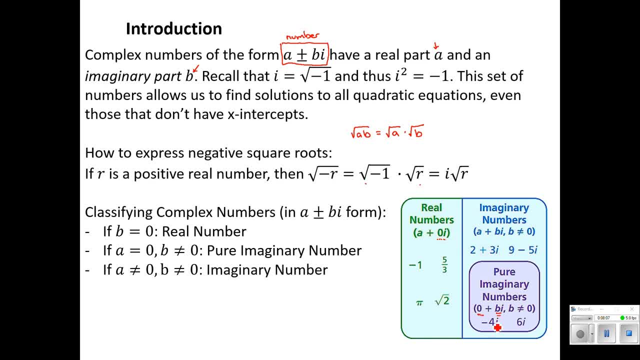 So these numbers simply look like something I And then, lastly, just a typical imaginary number is one that has a real part and an imaginary part, But again, these are just numbers. Even though they look like expressions, they are just numbers. 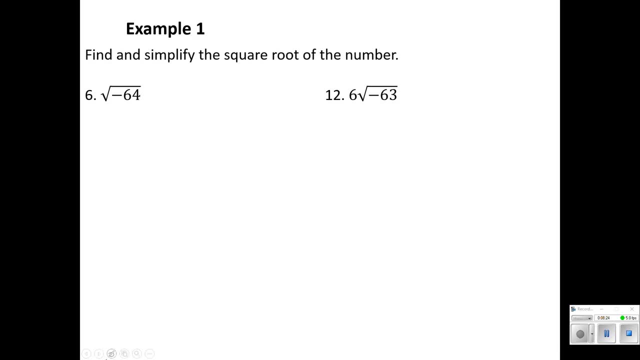 All right, So now that we've expanded our number system, let's use it. Number six: here we've got the square root of negative 64.. I don't like that negative sign underneath the square root, So I'm going to refer to that as the square root of negative one times the square root of 64.. 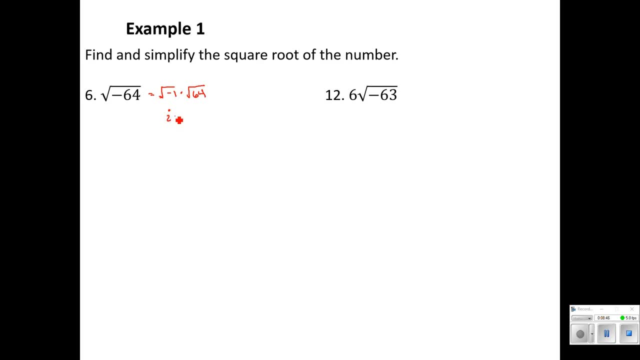 And the square root of negative one is I And the square root of 64 is eight. Now notice they were not square rooting both sides As a means of problem solving. this means the positive square root of 64.. So actually my introduction. I should not have said plus or minus three for square root of nine. 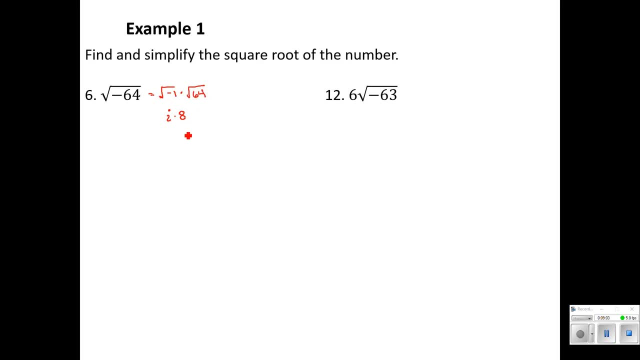 It should have just been a positive three. If anybody caught that, good for you. OK. so simplified imaginary number eight. I For number 12, same concept, except now there's a six multiplied out front. We just need to hang on to that. 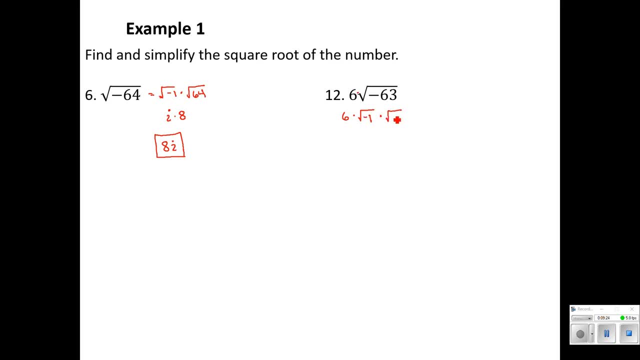 So I've got six times the square root of negative, one times the square root of 63.. OK, so I've got six I times And I just want to see if I can clean this up at all. So you may remember doing factor trees, where we try and break down a number through multiplication. 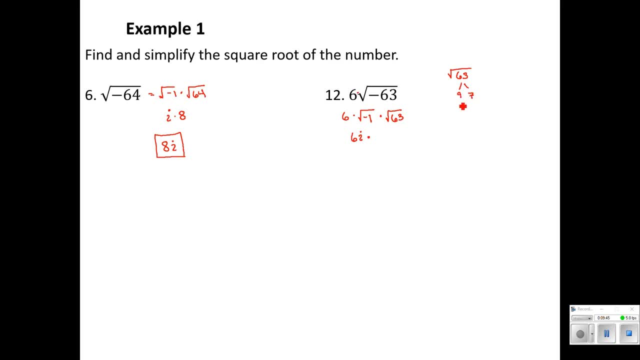 Sixty-three is nine times seven, And nine can break down into three times three. So now at the end of the equation, I've got six times the square root of negative, one times the square root of 63.. And now at the end of the branches of our factor tree, we've got a pair of threes and a lone seven. 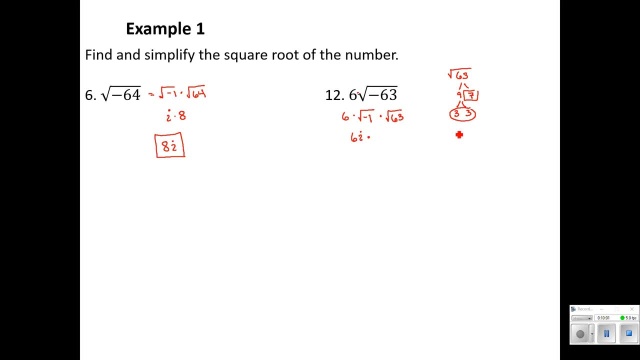 And what this is saying. I think a lot of teachers just say: oh, if there's a pair, then move that out front, And if there's not a pair, then leave it underneath. Well, why? Why does that make sense? 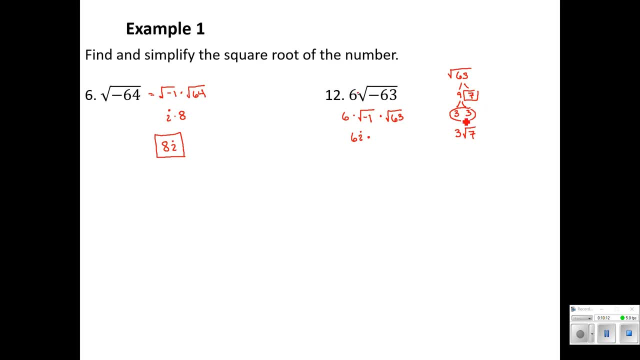 So just a quick explanation here: Underneath we've got three times three times seven. So what we've really done through our factor tree is set up three times three, That's three squared, That's three times seven. And remember, multiplication under a radical can be split up. 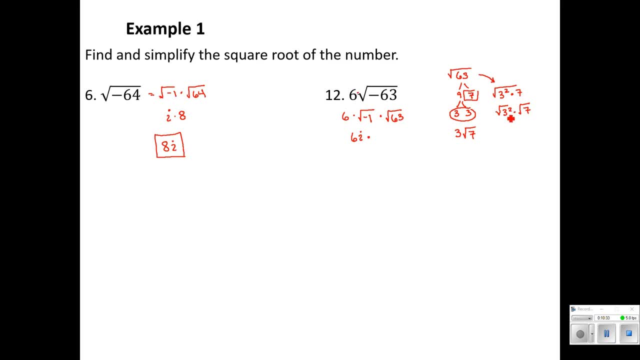 So this first part is the square root of three squared- Oh, that's just three. The square root and the square cancel out. That doesn't happen with the seven. So you can see why we look for pairs to free, But if it doesn't have a pair, then it stays underneath. 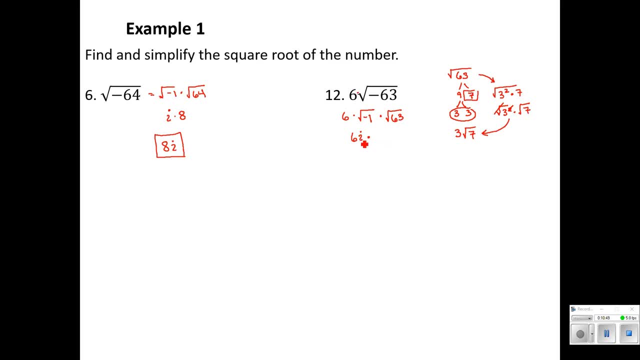 All right. So we've got six i times Three root seven. and again think about what this means. Six times i times three times root seven. We can clean that up. The six times three will be 18 times i times root seven. 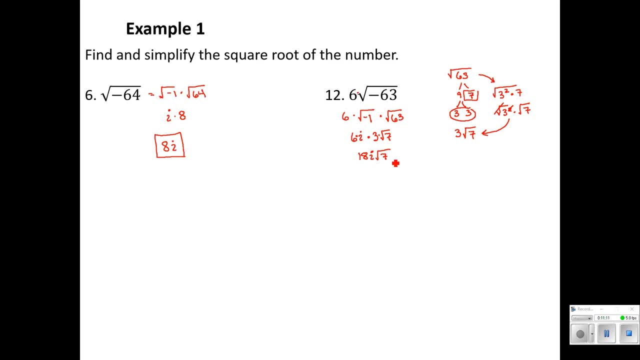 Now I know what you're thinking. Why is the i in front of the square root? Well, it's just so we don't confuse that as being underneath the square root. So if we have an imaginary number that has a square root in it as well, we typically write the. 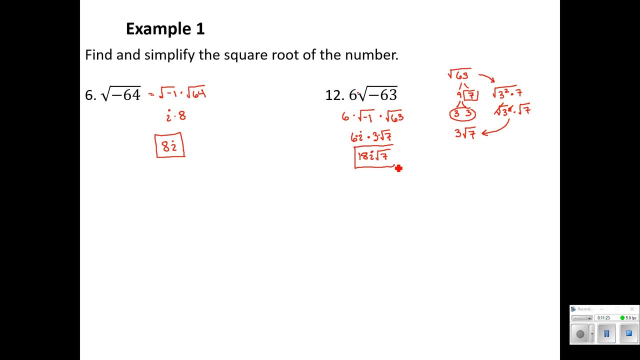 i out in front of that square root. So there you have it. Quite a bit of information in that slide. I hope that that makes some things clear that maybe weren't before. Our second example: find the values of x and y that satisfy the equation. 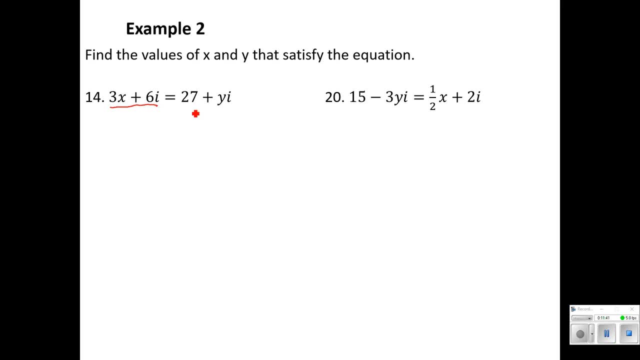 So here we've got this imaginary number which equals our complex number, which equals this complex number. Well, if the two numbers are going to be equal, that means they're real. Their imaginary part has to match and their imaginary part has to match. 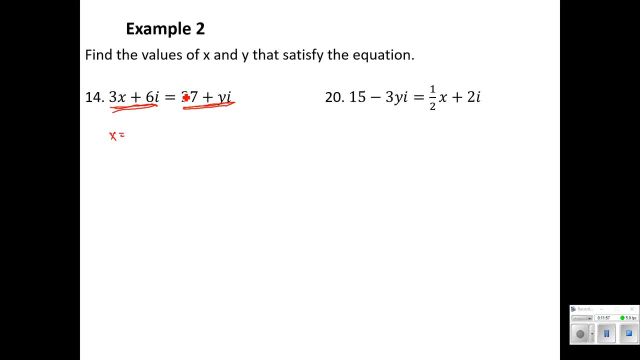 So to find x, I'm just saying, hey, I want this three x to equal twenty seven. What must x equal? So if I want three x to equal twenty seven, x has to be nine. and the same thing with the, the imaginary part here. 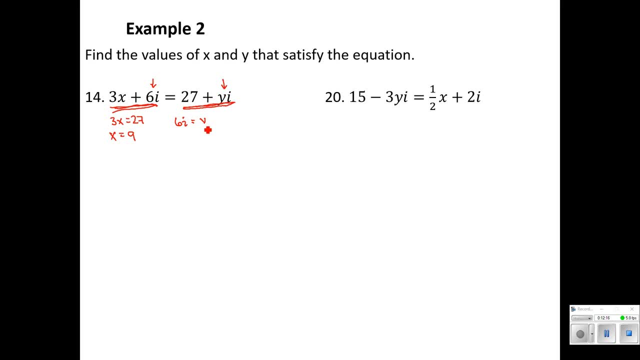 We want positive six i to equal positive y, i, Y, iota. Well, if that's true, then we're good. That's going to be true. Y has to equal six, And that was pretty easy to spot. Let's try the next one. 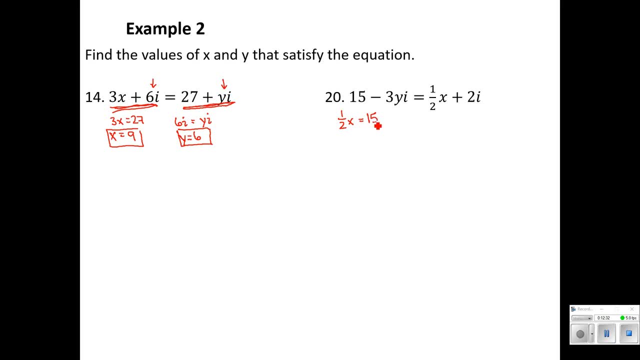 OK, our real part, one half, x, has to equal the real part in the other number. So multiply both sides by two. X has to equal 30. And in the imaginary part, negative three, y, that has to equal positive two. right to make the coefficient on the i term match up. 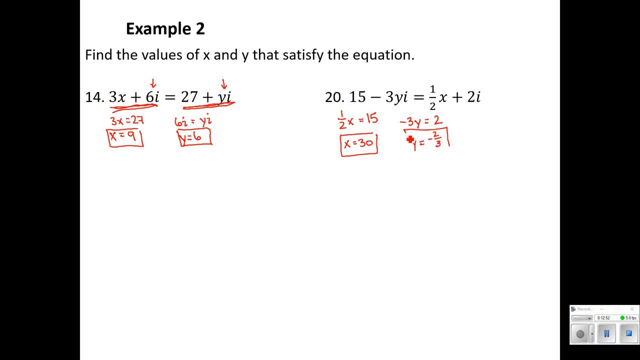 So y equals negative three. y So y equals negative three. y So y equals negative three. y So y equals negative two thirds when we divide both sides by negative three. So really simple. once we get it set up, You could say that was for a lot of mathematics, but really just kind of solidifying the idea that these are numbers. 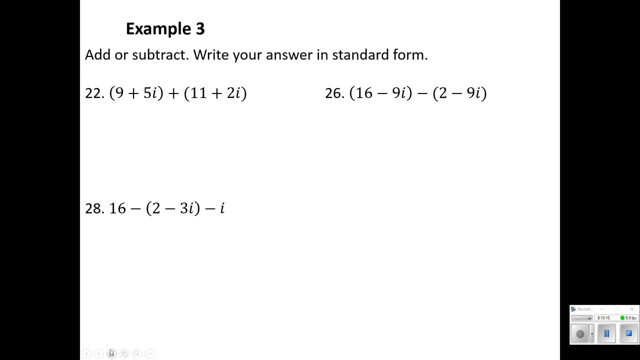 So they have to match perfectly. All right, Working with imaginary numbers. Now again, this is kind of reinforcing the idea that we have to match perfectly, So that imaginary numbers are complex numbers, They are numbers. So for 22, we're taking a number plus another number, one number plus another number. 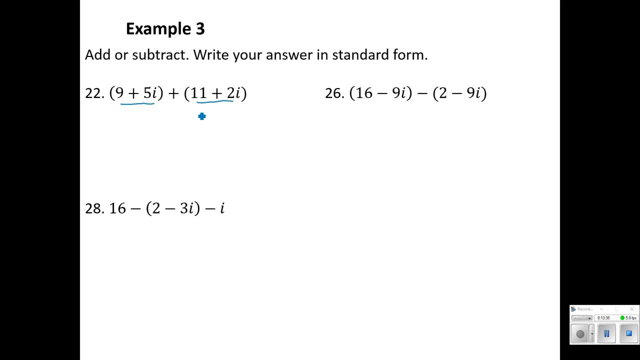 We should get a new number. We shouldn't end up with some fancy expression or anything like that. We should get another complex number. Well, all we do are combine like terms We can treat. i like a variable here, even though it represents square root negative one. 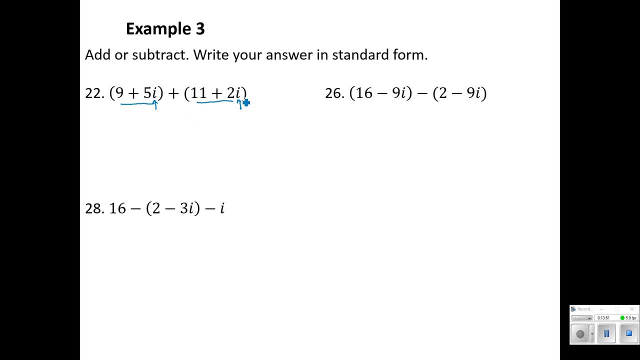 That property holds, So that's a good thing. So we can treat it as a variable throughout the whole process. So if we are just adding or subtracting, it's a matter of combining like terms. So I've got a real part of nine plus another real part of 11.. 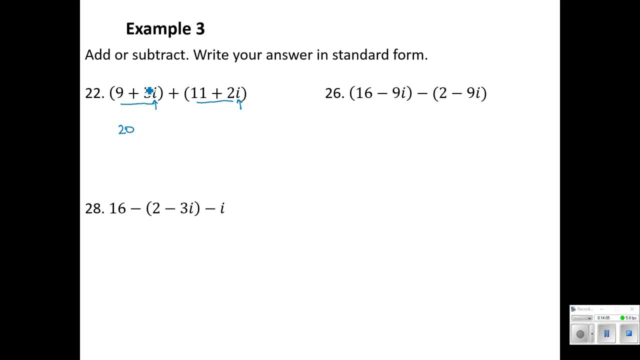 That's a real part of 20.. I've got positive five i for my first imaginary part, positive two: i for the second imaginary part. If I combine those together I get seven i For 26,. the process stays the same for subtraction, except now. 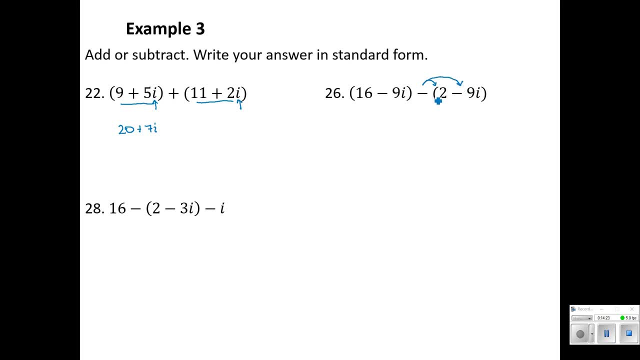 Just as if these were expressions, we distribute that negative minus two plus nine i, So 16 and negative two is 14 for the real part. Negative nine i and positive nine i gives me plus zero i for the imaginary part. Oh, that is a nice clean 14.. 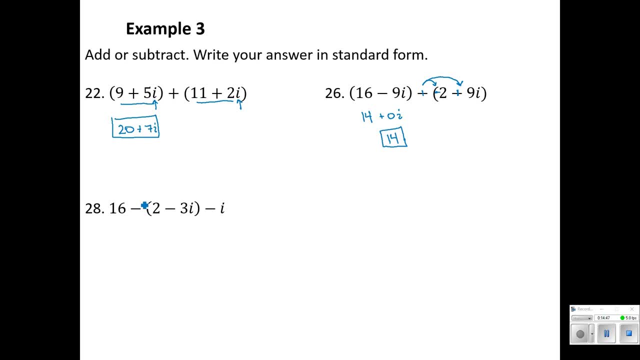 I can box up that other solution, 28. here again, more distribution. It's just following the original. So I've got minus two plus three i. when I distribute that negative, Let's combine the real parts: 16 and negative two is 14, positive three i. minus i is plus two i for the imaginary part. 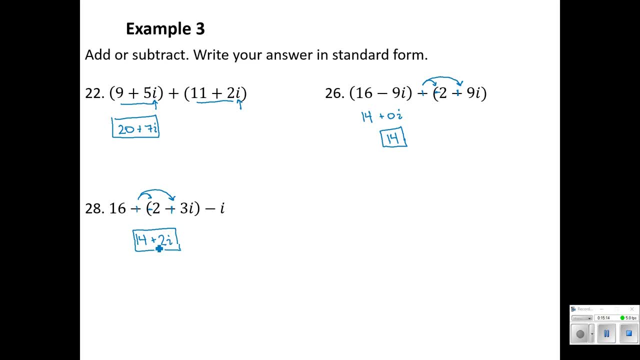 Now it looks like we could like factor out a, two or something like that. You do not need to do that. This is a number and that is our final answer. We don't want to distort that at all, So just leave it as it is. 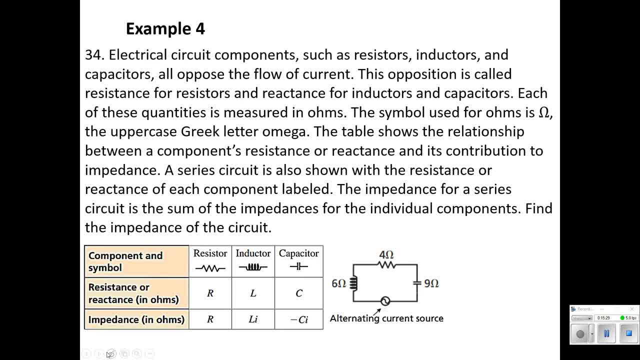 Oh boy. Example four: the literature lesson here, And this is a good example. Often you will see word problems in math that look incredibly intimidating. Don't be intimidated by the words So much of this is just fluff, and they really talk us through the process here. 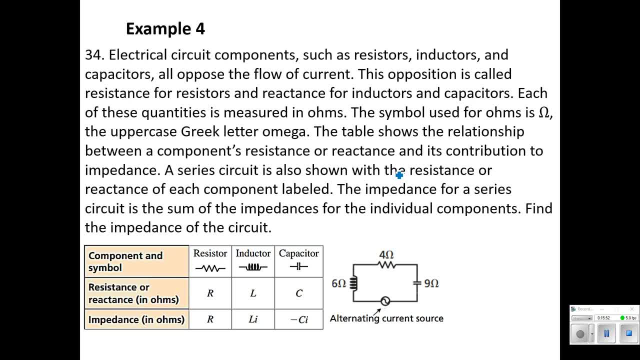 So take the time, read it carefully. It's a good lesson for all word problems. I know a lot of students will look at this and just say nope and shut their textbook. Don't be that person. Invest a little bit of time, read the problem and give an honest attempt at it, because if we can interpret this, 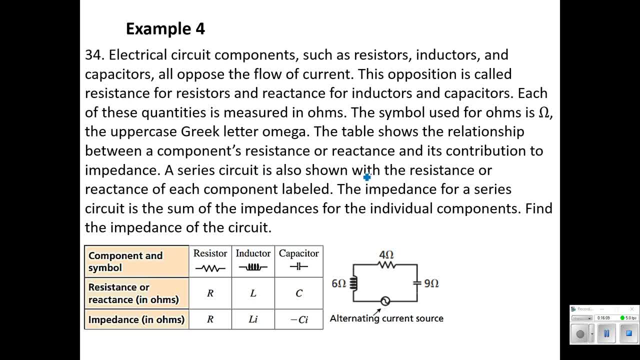 and come up with a reasonable means of solution. we're going to keep growing and becoming a better math student. All right, here we go. Electrical circuit components such as resistors, inductors and capacitors. We do not need to know anything about electrical circuitry here. We're not. 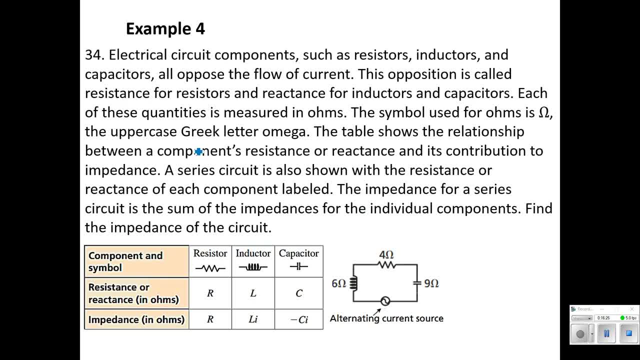 electrical engineers. They're just explaining this concept. This opposition is called resistance for resistors and reactance for inductors and capacitors. Each of these quantities is measured in ohms. The symbol for ohms is the uppercase Greek letter omega. The table shows the relationship. 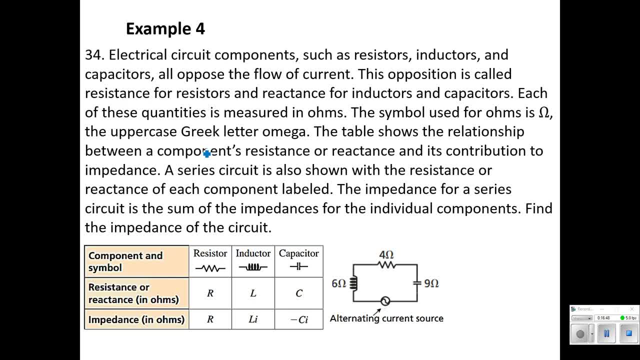 between a component's resistance or reactance And its contribution to impotence. A series circuit is also shown with the resistance or reactance of each component labeled. The impotence for a series circuit is the sum- there's our first math word- of the whole process of the impotences for the individual components. Find the impotence. 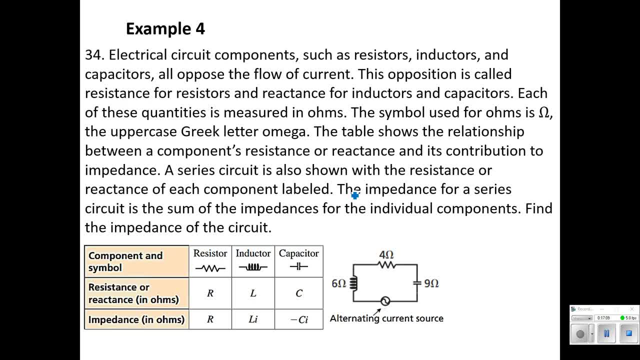 of the circuit. So really everything except for the last two sentences is irrelevant to what we're trying to do. Okay, so find the impotence of the circuit. So really, we are just looking here And we want to take the sum of the impotences of each component. 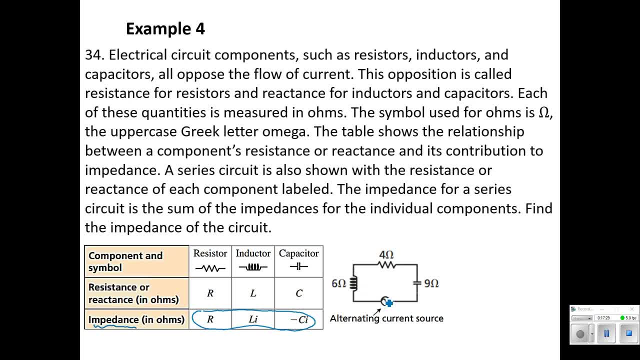 of our circuit. So our power flows from this alternating current source and then it goes through an inductor- right, We can see the coil. so we match that up in the table which says Li. Okay, well, L is just the coefficient there. So we've got six I, and then we've got 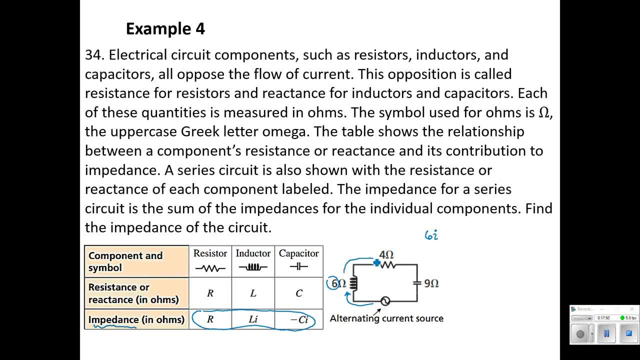 four, I All right. and then we want the sum, so our current keeps going through. Then we get to a resistor Notice. that is just R, That's just the number. There's no imaginary component to it, So it's just four. 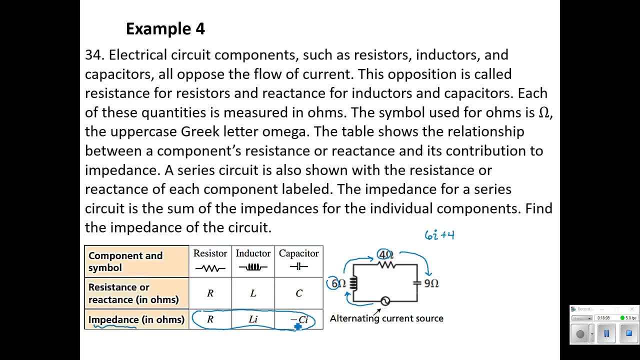 Okay, then we keep going and we finally get to a capacitor which is minus Ci. So here's this: nine, That's our C value. So minus C, nine I. That's it. That's all they want us to do. Sum of the components of a circuit. 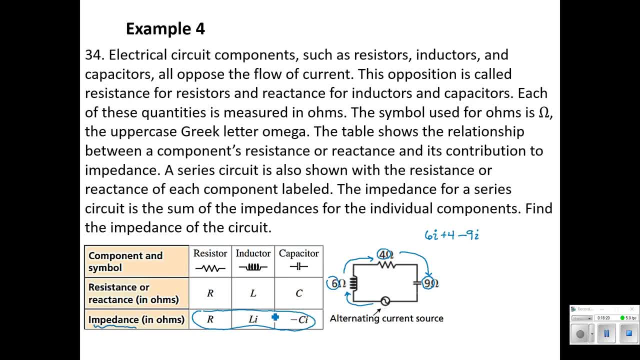 those components and put i's where they need to go And if we combine that together we get 4 minus 3i for the impotence of that whole circuit. Very, very intimidating looking problem, but look at how little work that took to. 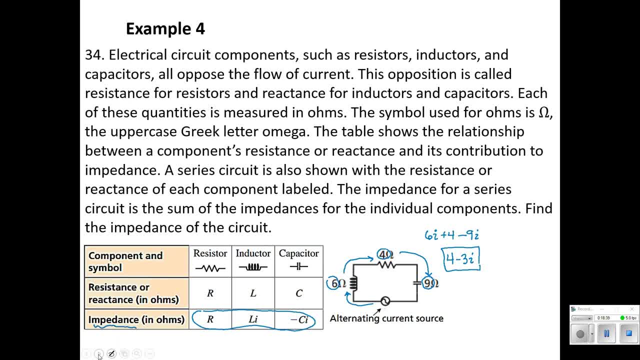 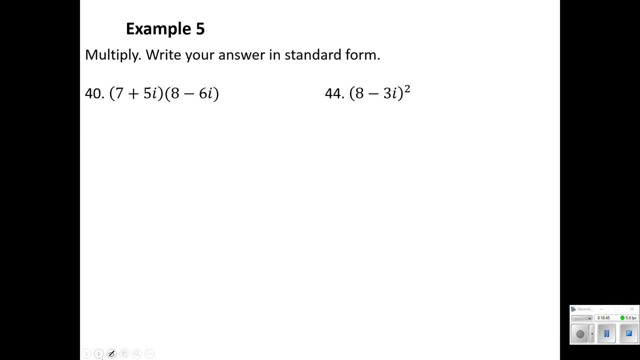 actually write out and solve that problem. So again, take the time and put an honest effort into these word problems. you'll definitely reap the rewards of that later on. Alright, example 5,. now we're multiplying and, just like before, if we took a number times a number, we should end up with a number. 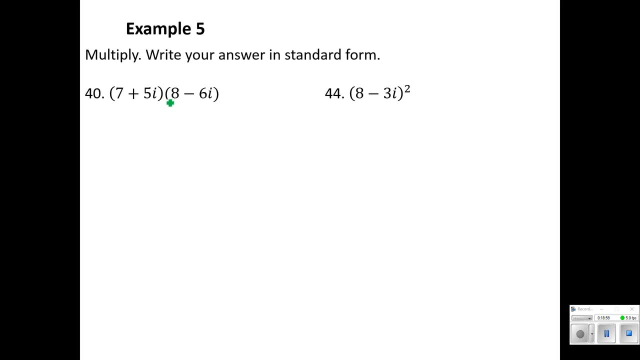 for a result. So we don't want to see anything that resembling a function here. we want a nice number that's following our a plus or minus bi format, a complex number as an answer. Now, even though these are not expressions, they're numbers we can certainly treat. 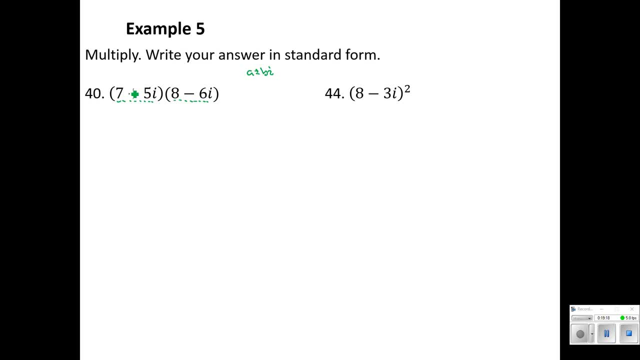 them as expressions, And if you know I were to give you this without any directions whatsoever, I would hope that you would start to FOIL them out First times. first, 7 times 8 is 56.. Outside, we got minus 46i, inside, I've got plus 40i. 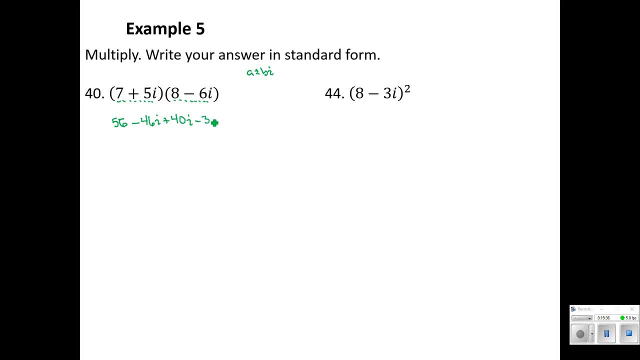 and last times, last, I get minus 30, and there's an i times i in there. i squared Alright. well, the way I want my answer to be, there's no, i squared in there. so we need to find a way to reconfigure that. Remember: i squared is really saying the. 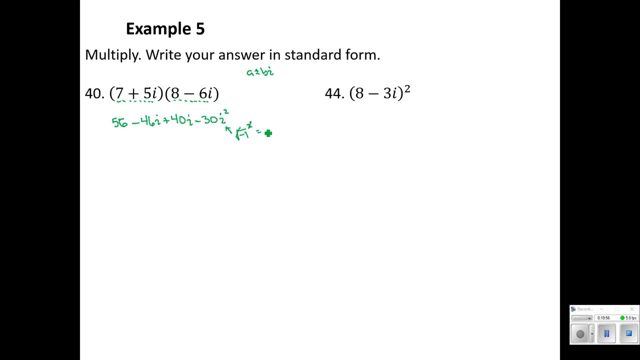 square root of negative 1 squared, so i squared is really a negative 1.. So I could think of this as 56 minus 46i plus 40i, then negative 30 times negative 1 plus 30. Now we can combine our like terms. We get 86 minus 6i And you can see our answer sure. 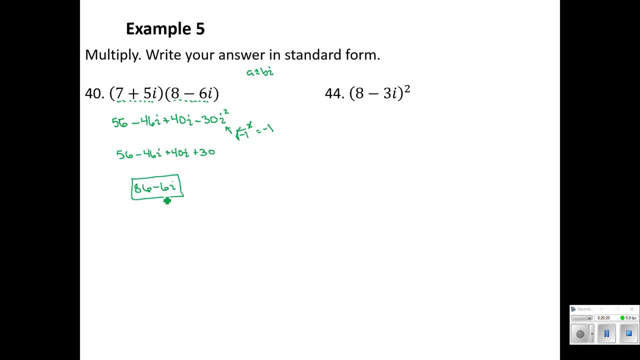 enough. it's following that, a plus or minus bi format. That is a complex number. as an answer On number 44,, we may have talked about this in class. We may not have One of my life hacks for math. there are so many times where you need to take what looks like a binomial. 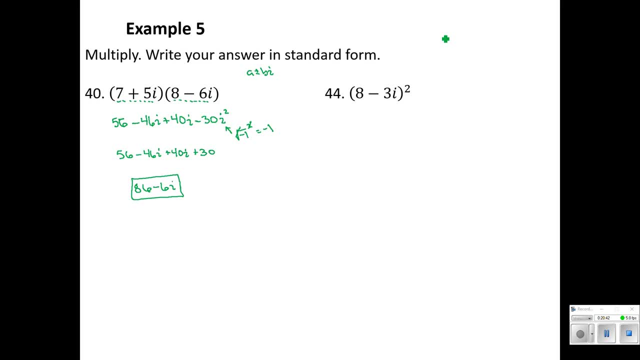 a simple expression like this and sort it up, Here we go. I do like this. If i put square it, This is: you probably learned something like this in eighth grade math class. but if we have something of this form and we are squaring it to streamline the foiling process again, 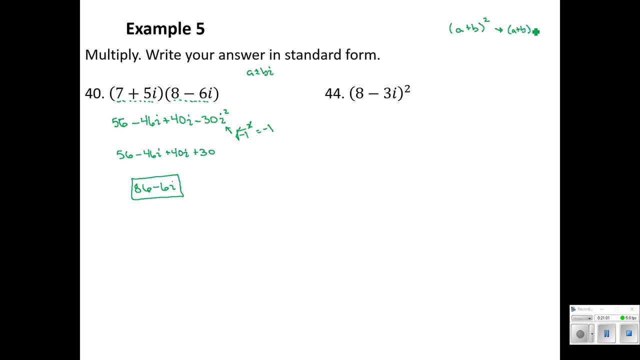 what it's really representing is a plus b times itself. That's what squaring means, And first times. first would give me a squared, outside would be a b, inside would be another a, b, and then last times last is b squared. So I'm not often. I don't like to condone memorizing. 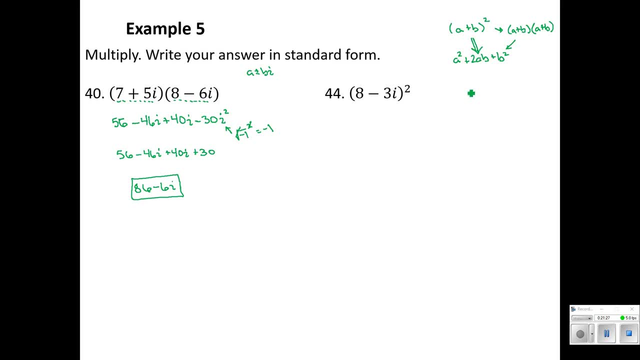 often, but if you can remember this simple pattern, it will make you a much, much more efficient math student. You don't have to, but it does speed things up greatly. So let's try that here in this example, and if you latch onto it, excellent. but if you don't. 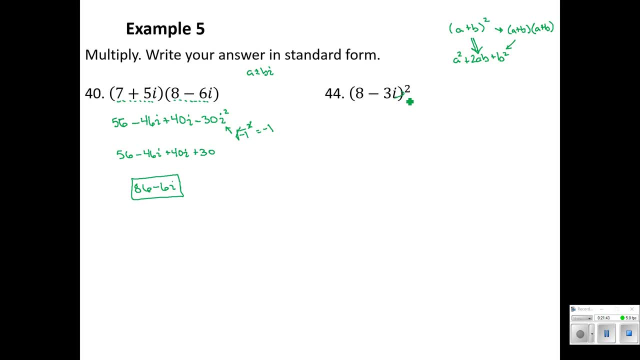 don't worry, you can always foil this out. Just remember that we need to do the foil method here. So 8 minus 3i, that quantity squared- I do first thing- squared 2 times the first, times the second. 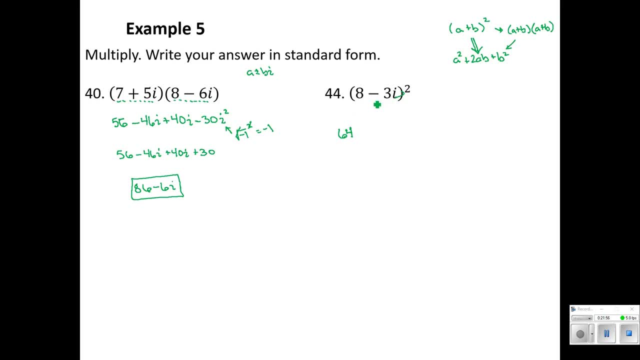 2 times, 8 times negative: 3i. 16 times negative 3i. that's negative 48i. and then the last thing squared. So that's the first thing squared. So that's the first thing squared. So that's the. 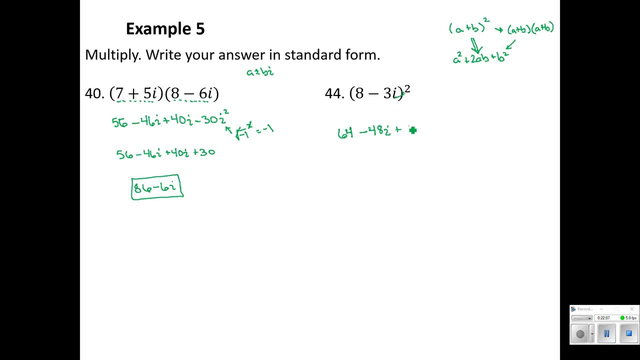 second thing: squared, Negative 3. squared is positive 9, and we got to square the i as well. Now remember this: i squared is meaning negative 1, so instead of plus 9i squared, it's actually minus 9 when we simplify that i squared, So I end up with 55 minus 48i. for my final answer: 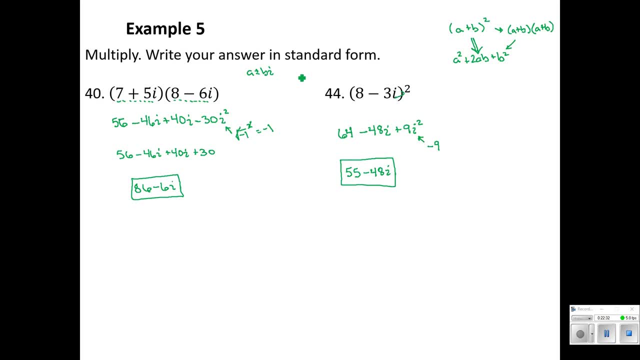 That's what we should expect. right, We're taking a number and squaring it. We should end up with a number. Okay, example 6, solve the equation. So we talked about in chapter 2 several different equation solving techniques, or maybe it was just section 3.1, actually that we went through that. We've 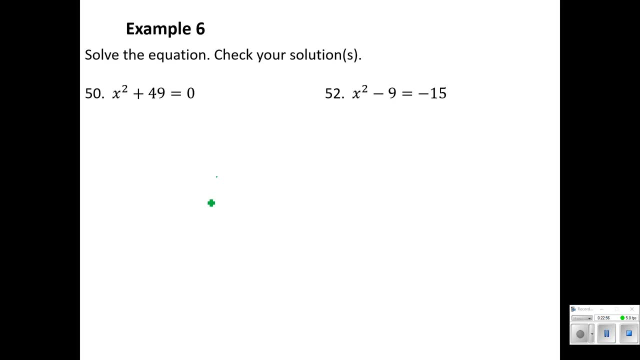 got factoring. we've got the square root method, but here you can see number 50, we got x squared plus 49 equals 0.. I've got my variable squared. There's no other x terms, so I don't need to factor. Let's isolate that x squared and then we can solve by square rooting both sides. 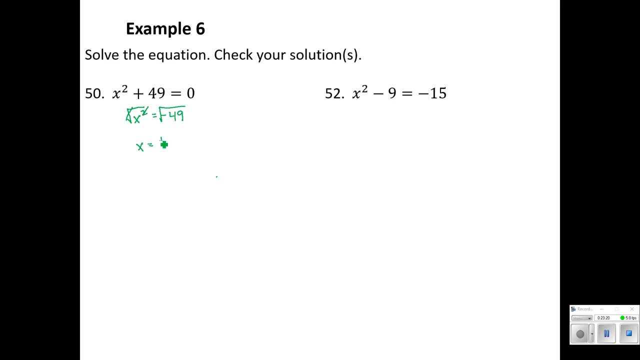 Now we're taking the square root as a step in problem solving. so that's plus or minus, and then square root of negative 49 is like square root of negative 1 times square root of 49.. Square root of negative 1 is odd. 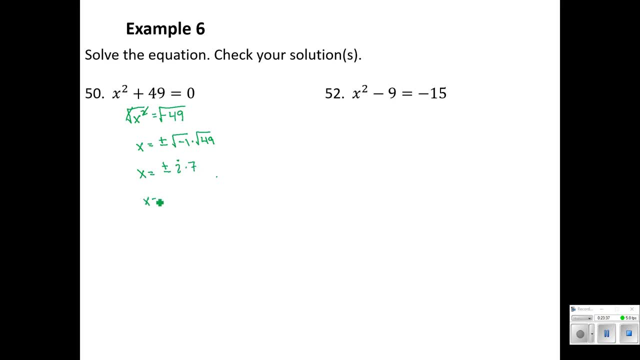 I square root of 49 is 7,, so my solution is plus or minus 7i. All right, now you don't have to go through all of these steps. This is just to illustrate the thought process that should be occurring in your head, but I know right away that many of you will be able to set this up and come up with your solution pretty quickly. 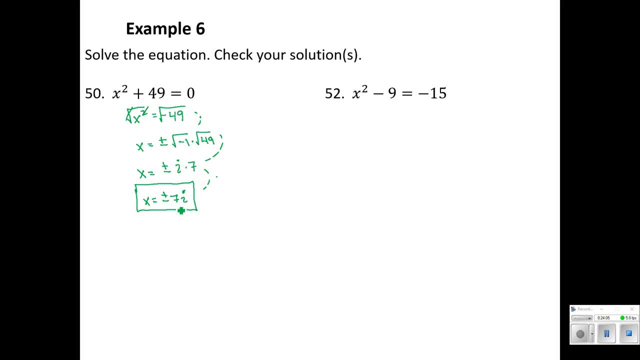 So don't feel like you have to show all those steps. All right, now we're supposed to check our solution. Well, what that means is I'm going to take 7i squared plus 49 and see if that equals 0.. 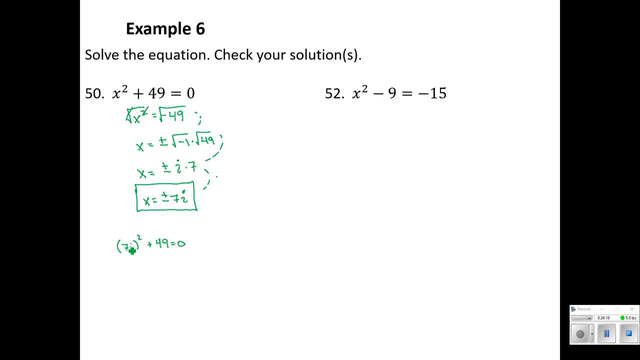 Test it in the original equation. Well, if I square 7, I get 49.. If I square i, I get i squared, which is negative 1.. Is that a true statement? Yes, that'll be negative. 49 plus 49 equals 0.. 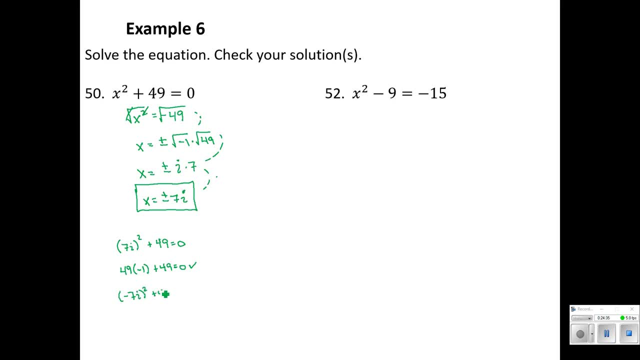 What if I did negative 7? I squared. Does that one work? Well, negative 7 squared is 49, and then i squared is negative 1, so we get the same result. Good, so our answer checks out 52,. here we've got some more set up. 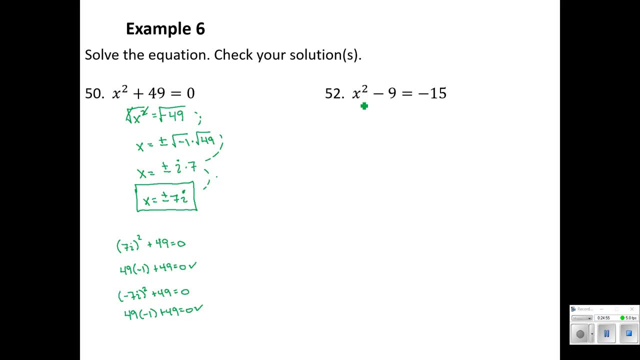 You can see again no x terms. so we are good to use the square root method. Let's add 9 to both sides And then we're good to square root both sides. So x equals plus or minus square root of negative 6, which is root negative 1 times root 6.. 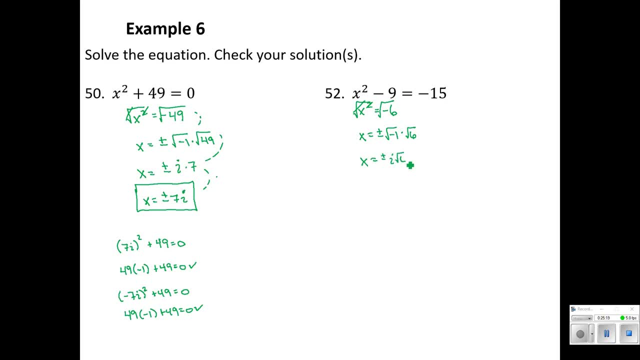 So x equals plus or minus. i root 6.. Okay, that's the solution we arrived at. We cannot simplify the 6.. If we wanted to try a factor tree, you can see no pairs are made up when we divide that, radicand out as much as possible that 6.. 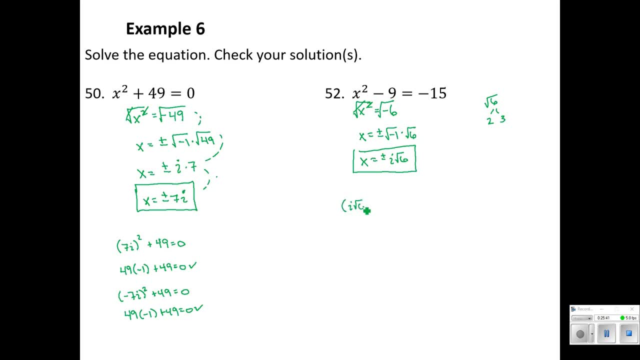 So let's test it out. i root 6 squared minus 9, does that equal negative 15?? If I square the i, I get negative 1.. If I square the root 6, I get 6.. Minus 9, does that equal negative 15?? 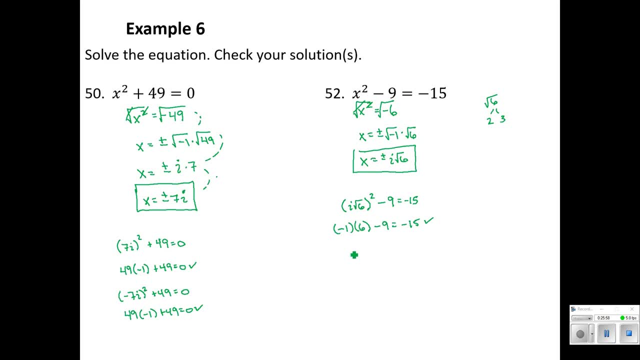 Negative 6, take away 9 more. You bet What about negative? i root 6?. All right, if I square the negative, i ooh it's like squaring a negative number. We know that's going to come out positive.